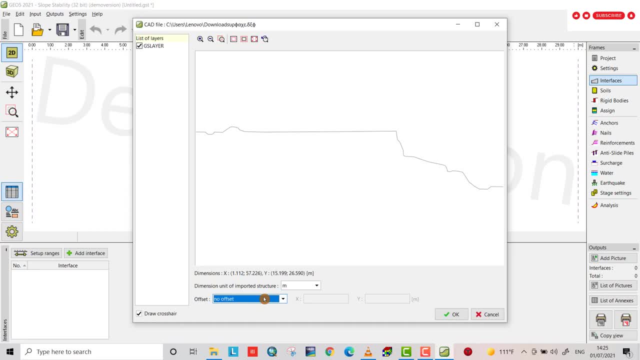 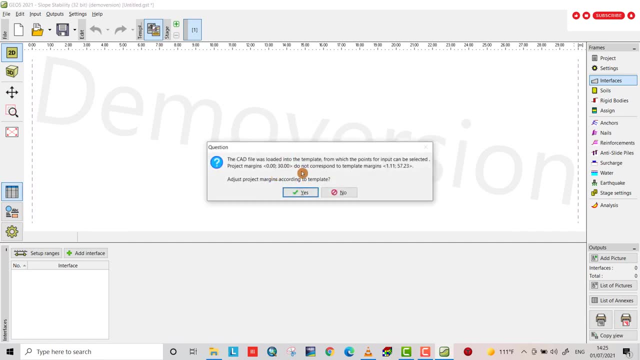 Otherwise it not be fit together, So that's why I choose no offset. OK, You see project margin 0 to 30 and do not correspond to template margin 1.11 to 57.23.. Adjust, Yes, adjust. 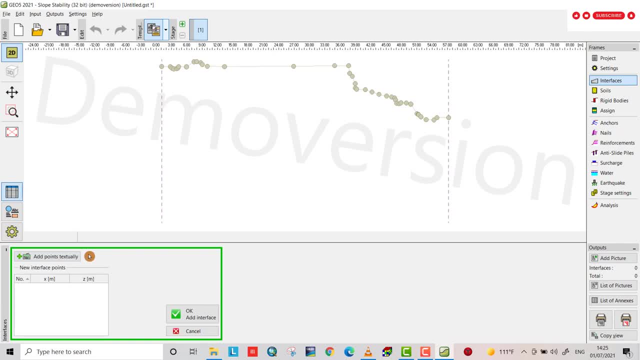 That is the point. We just draw the interface through these points. we have, OK, Add, Add interface. Add point No, not point Yes, Draw. You just go through the points. That is the surface of slope we have. 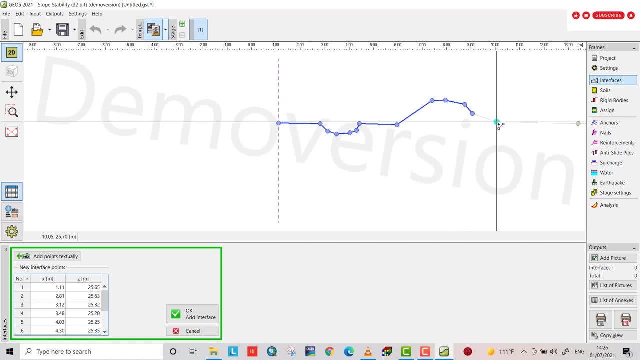 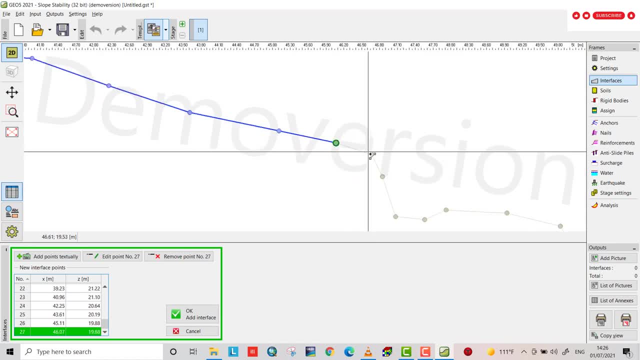 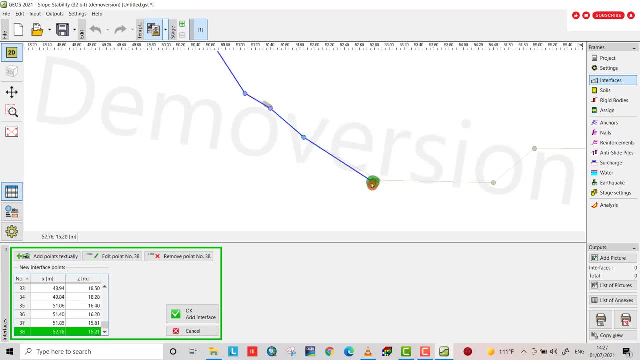 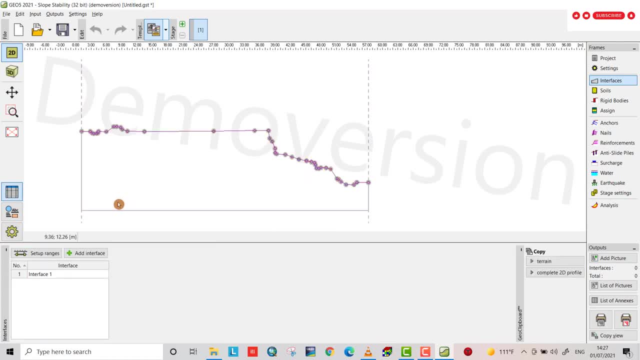 OK, OK, OK, OK, OK, OK, OK, any point that is, I choose from here. okay, that's the bottom of the test layer. okay, also at another interface you can also provide the layer by point is textually. but first we have to know. 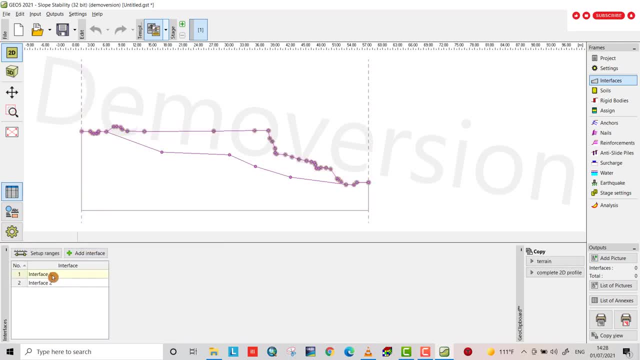 where is what is the coordinate of the first point? you see, first point is one point 11, X and 25.65, is it? so it's a good information for us to start at interface at points. textually, I choose 1.11 as X and 24 for that. you see, that's the first point and the 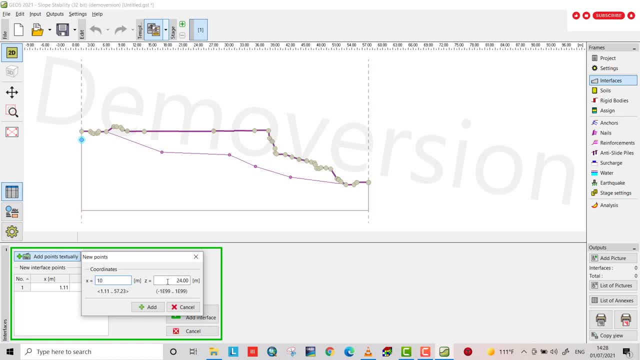 second, I choose 10, X and 23 for that okay. 20, I choose 20. okay. 40 X, 50 for not. let the 12. okay and 50 thirty, no. the last point: 55.23, 54.23 and should be. I should make it 11 or it be. 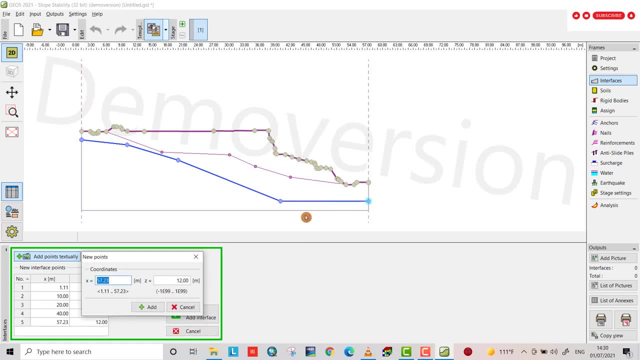 told: okay, that is also the way, all the sea ways to bring a, to draw a, the IBIS camera process to create a job. with all these steps, three or four is also possible and you can find many ways to realize the job with body when we just need a rough drawing process like this and those are: 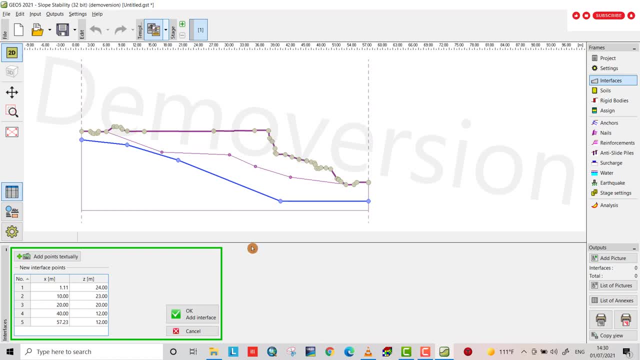 the section by the template or just drawing or just by putting the point. so when we have a point, just I want to show you how you input the section. okay, do you want to cancel? no, no, I'd interface. we have to define the solace for the. 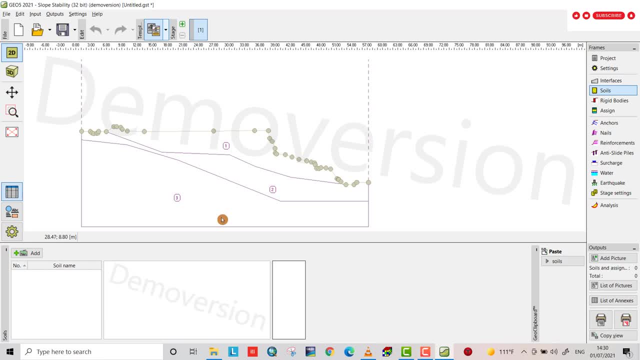 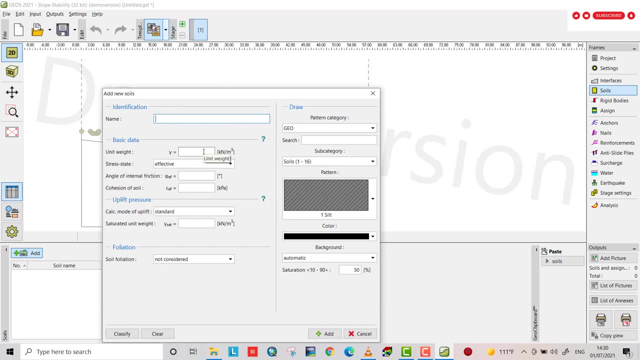 first tutorial about analyze and the design of separate footing. I put the data for the soil, but here I just choose the soil from the program because the job I do is different type of soil. so if you want to define the soil by yourself, you can watch my video. I put it in a description from: 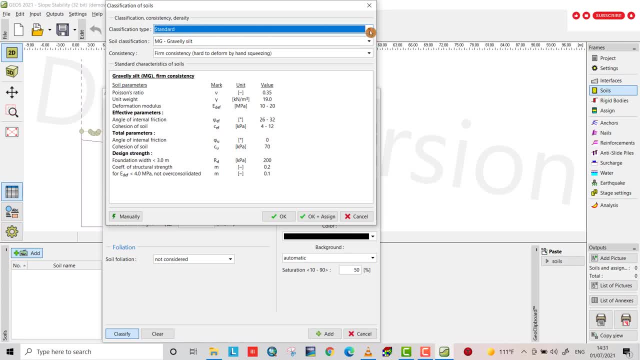 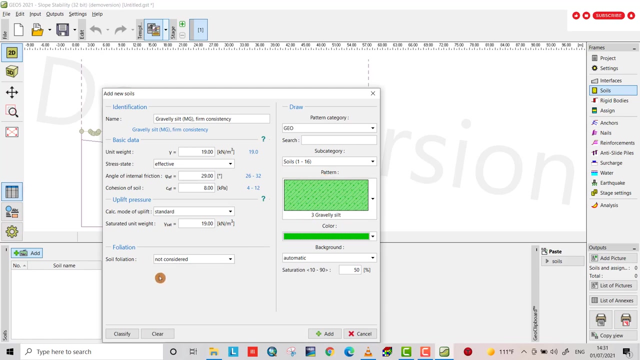 classification: you see, we have from classification type, standard and China, I choose standard. and that is a different type of soil. first soil: I choose gravely silt, gravely silt, okay, gravely silt, yes. and film consistency: I choose film consistency also. you can change the color. let's be great. you see directly, program fill all. 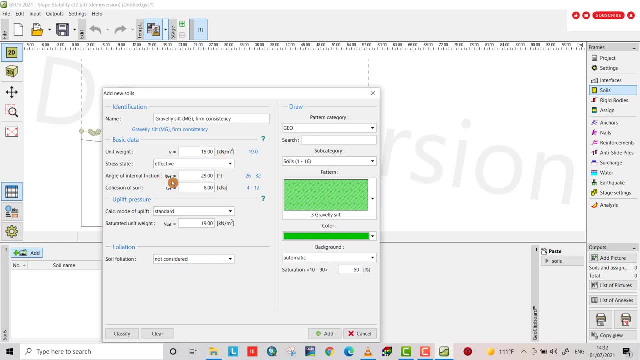 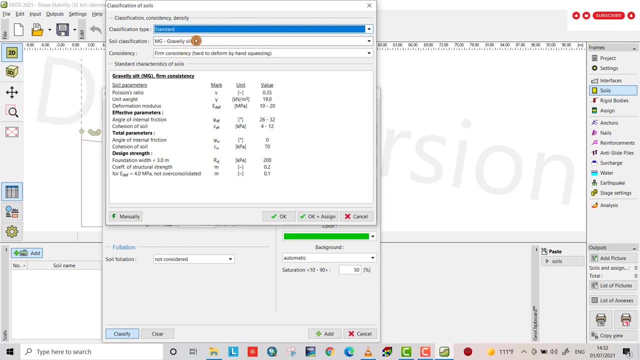 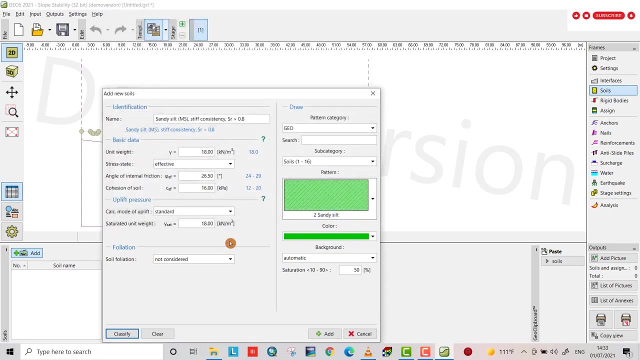 the gaps you see. for angle of internal friction there is a range: 23, 26 to 32. each is the program. choose the 29, you can change the data. okay. another one, another one I choose, see MLMI. I choose the bottom'll, okay, and you are. 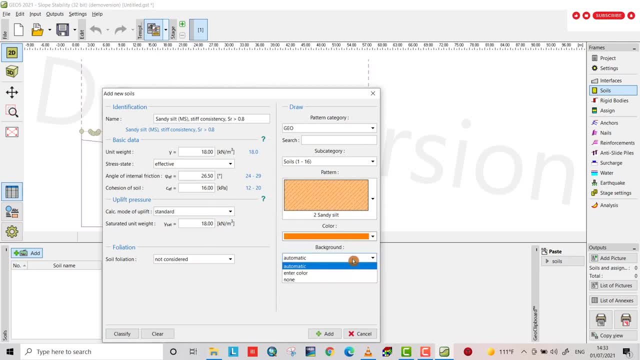 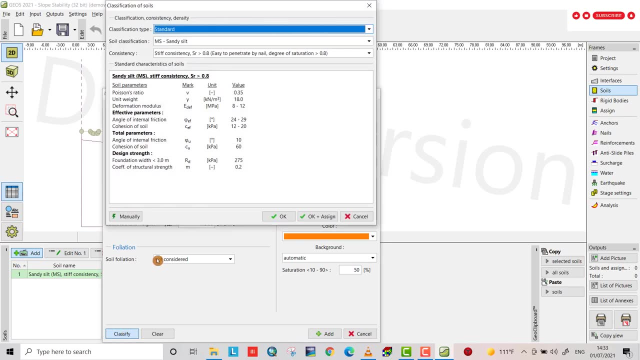 seeogo coreyn. all zones, those have always and one, so it's not for fl Ford, so let's enjoy the video. hey, all of you doing so good, you wish that you you've done this alone. let me give you some tips for for burning all oceans. soil 당신, if you like video. 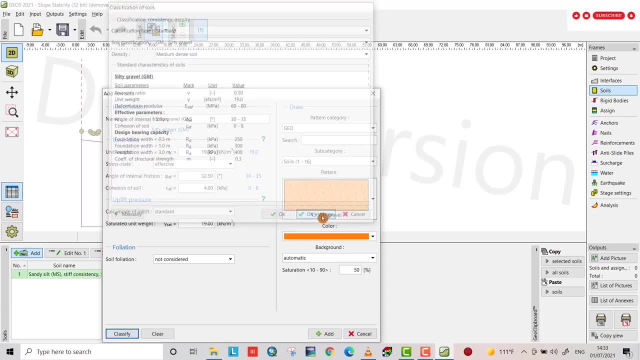 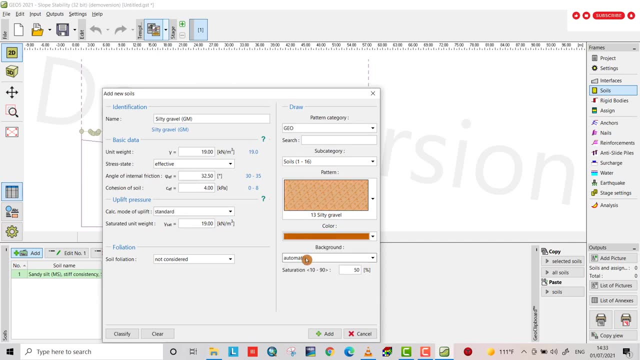 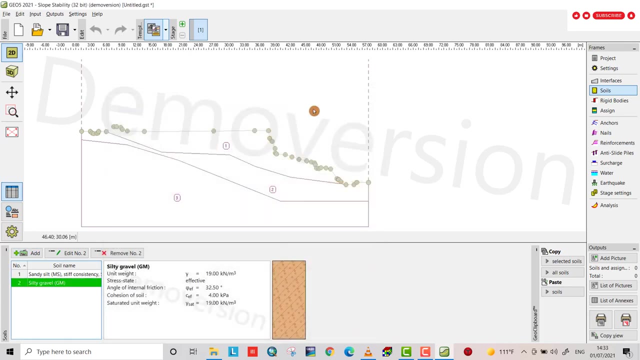 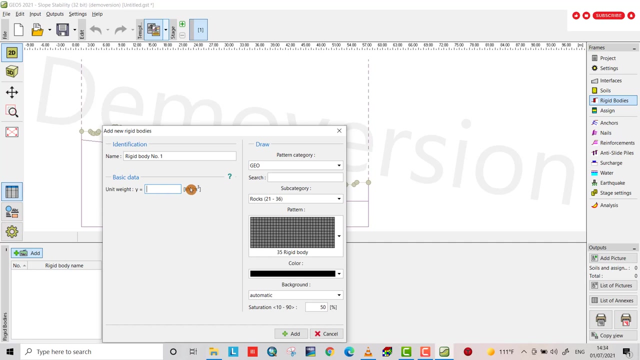 planning projects medium depth. okay, and sign and change the color at the this one. okay. now we have a different source. also, we can provide rigidbody rigidbody. there is no change in the rigidbody, just it provides the unit weight at the 21 kilonewton and the color at the black. okay. 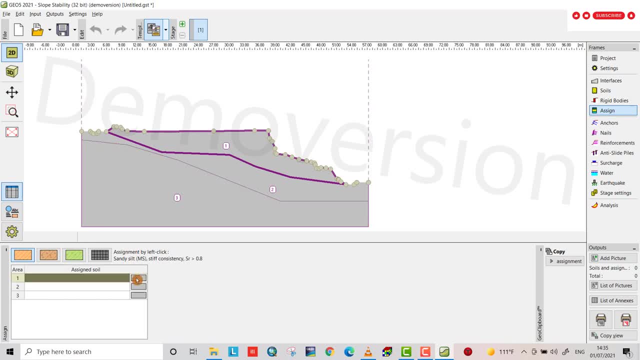 assign for faster. okay, grab the shield, yes. second there, provide silky gravel and for the layer you can still throw, provide circular. let's change the color now. safety cover, not this one. globally. still Sunday here. okay, I don't provide a rigidbody. if you have the rock, that so you can provide rigidbody, but I don't. 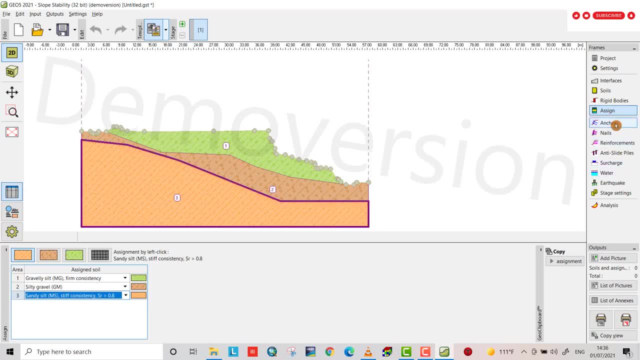 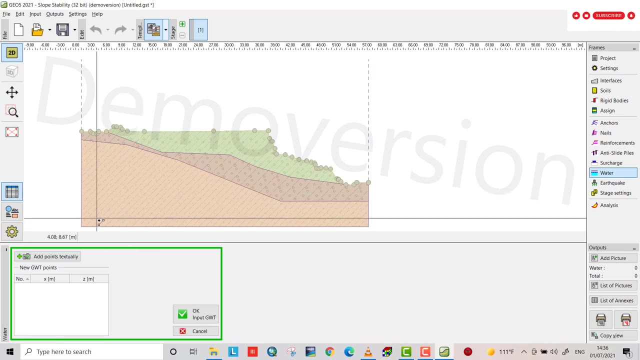 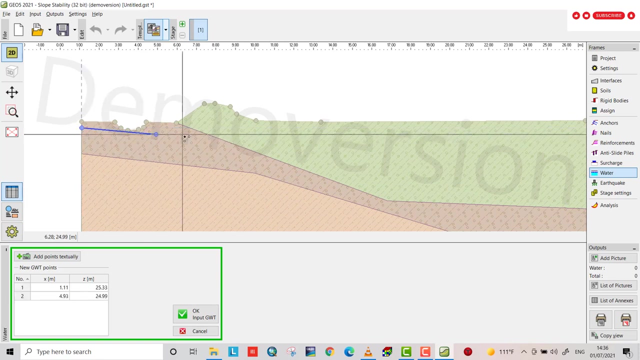 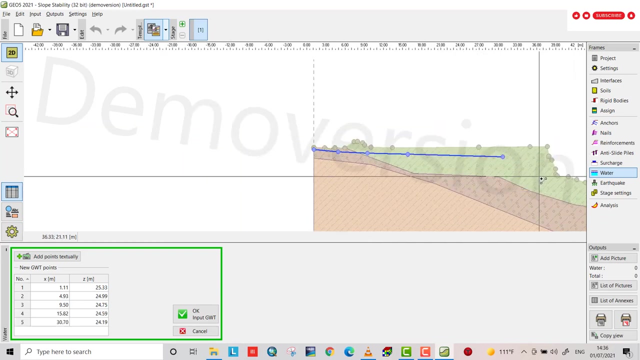 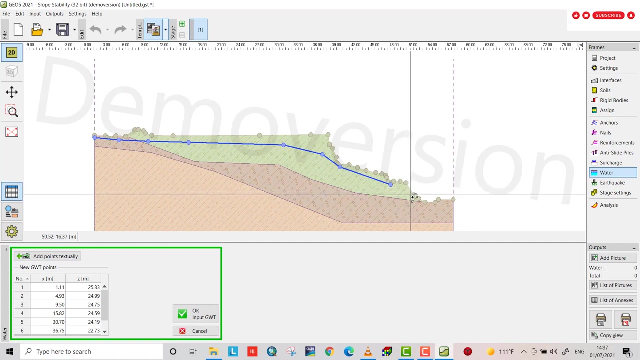 provide also on teres, Nellis and slides, their charge. in this stage I don't provide search at. in the next stage I provide search at. let's provide what table, okay, input ground, what table? I draw. you see you, this is what the 40 radius. 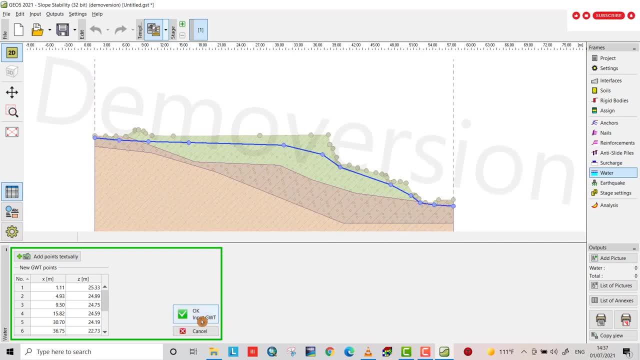 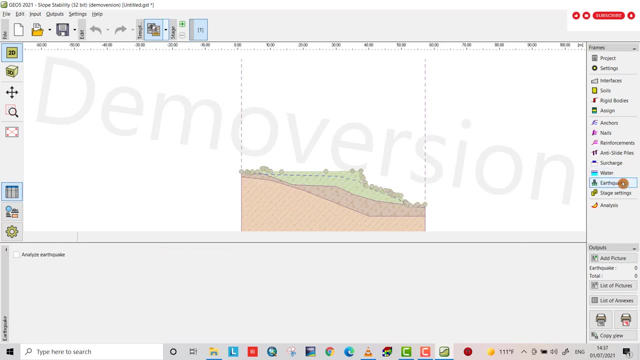 also can provide size system if you have a rather a tied below the scale and the ok uses. let's analyze bishop standard and also input graphically. i want, if you want, to find the slope stability for this section. okay, analyze, you see, it's not acceptable. 1.21 smaller than limit is the limit also. 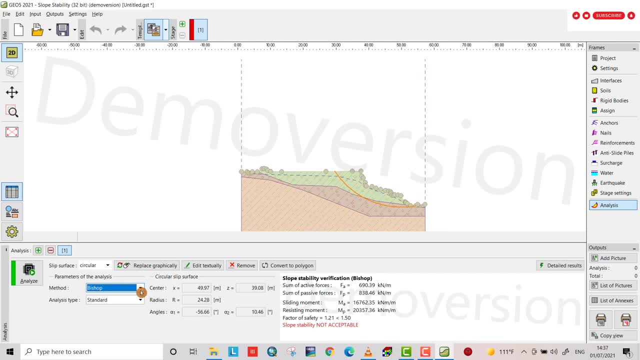 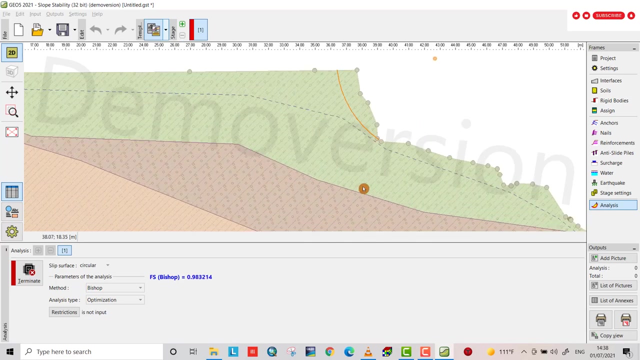 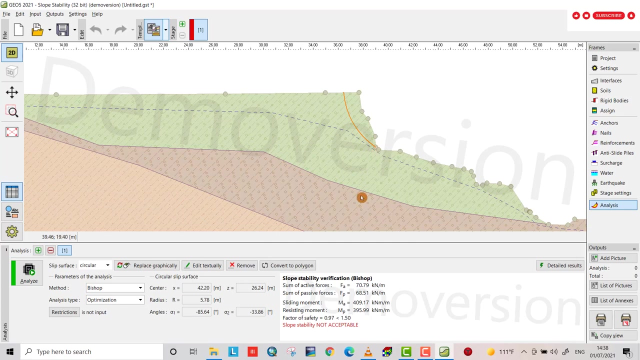 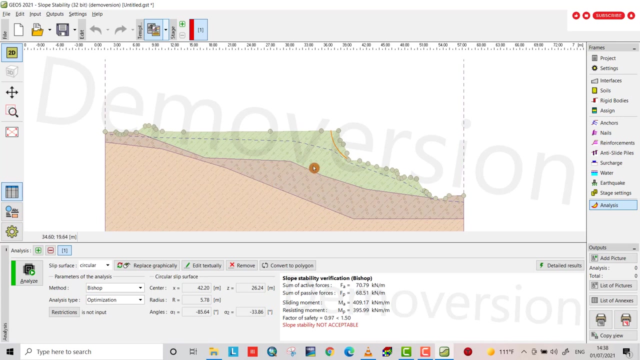 you can optimize to find the most weak slides. just use optimization. you see how the program optimize and finds the weakest slice. you see that is the weakest slip surface, which is 0.97. okay, also, if you have a weak layer, you can find the slope stability or factor safety for this slice by. 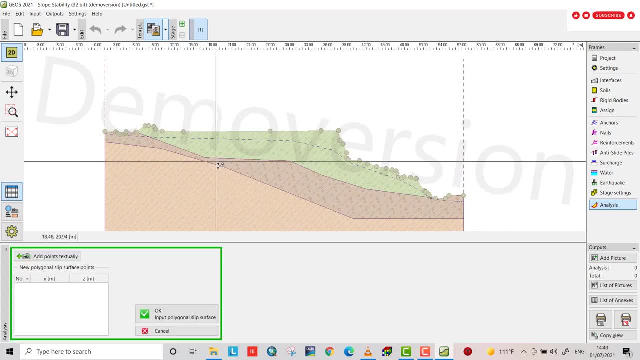 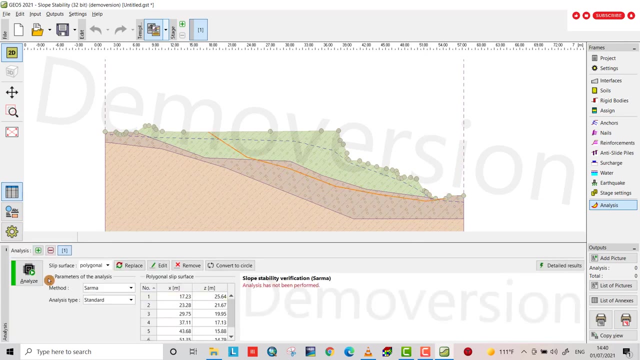 not by circular, by polygon. if we, if we check the uh uh stability of this section, okay, analyze it is over the limit, so it is safe. also, let us find some solution for this slope. stability for the stability, i'm sorry, yes, not circular. optimal addition provide, no, no, just analyze, cancel, just analyze. 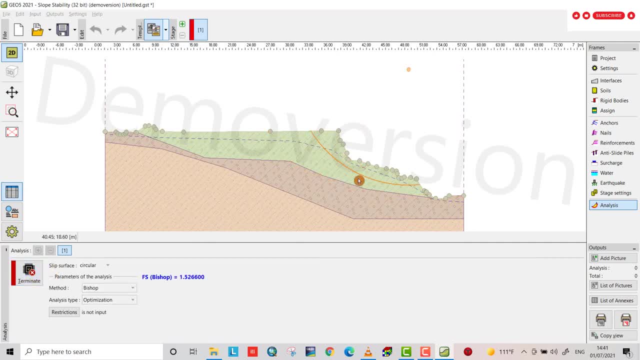 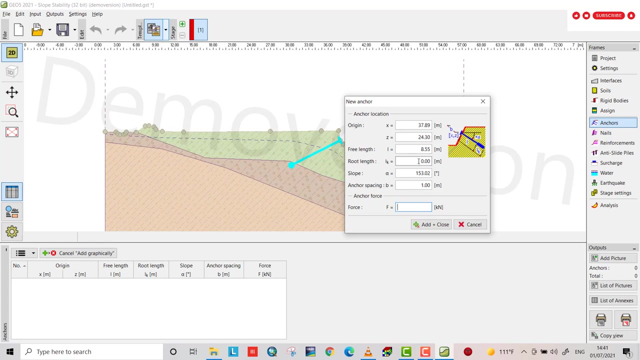 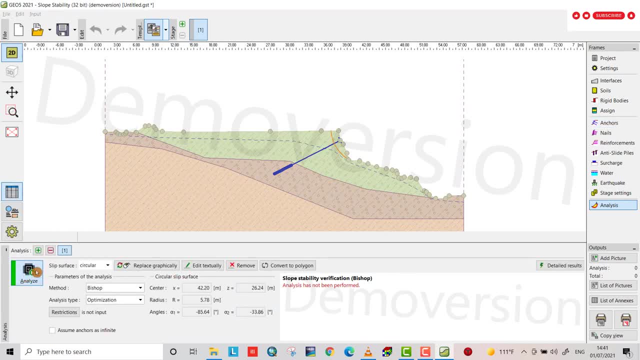 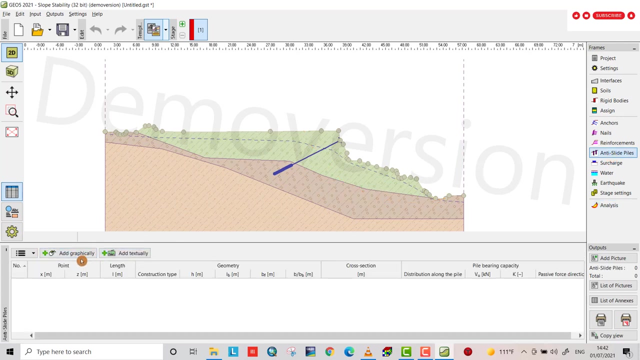 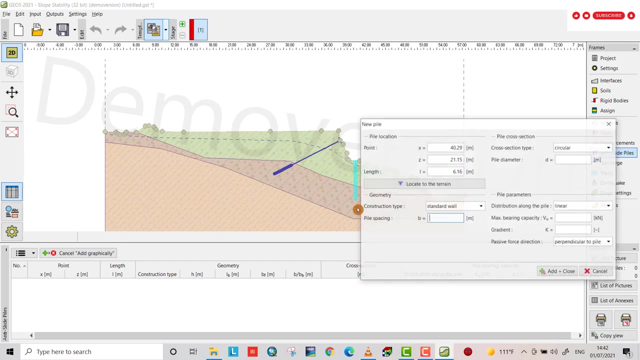 okay, let's provide it. analyze this time. you see, now this one is safe, but there is some problem here. 127, if we provide some uh 127, if we provide some uh. 127, if we provide some uh. anti-slide palace, okay, add graphically: fire space: one meter diameter, let be 0.4, bearing capacity, let be 100, sorry, 100- and gradient: 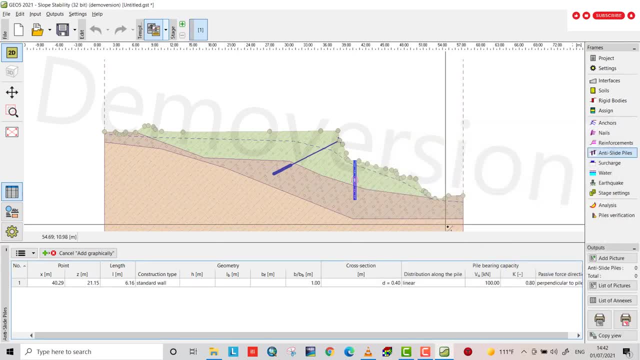 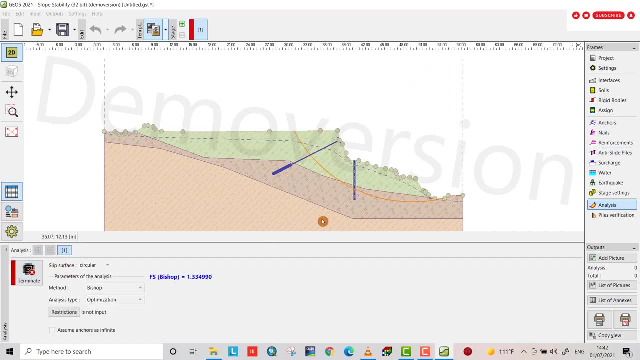 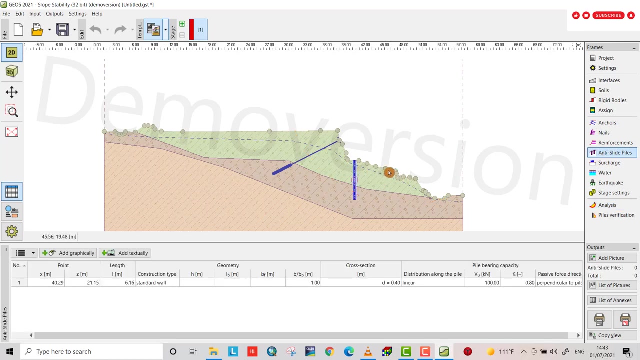 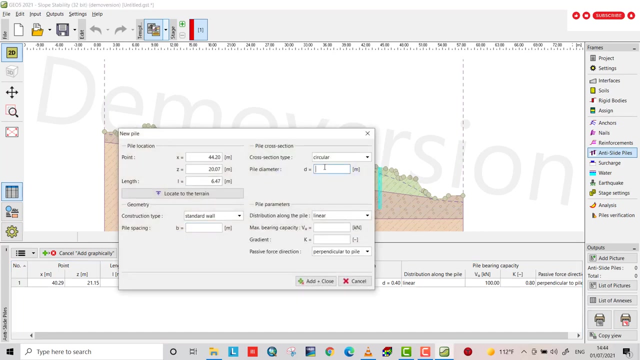 let be 0.8. okay, this time let's analyze and it's. you can't see any difference. you see it's 1.27, change it to 1.33. that probably write another anti-slide pile. no, sorry, add graphically d: 0.4. 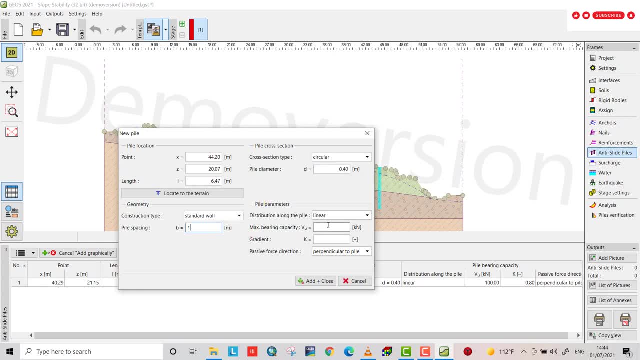 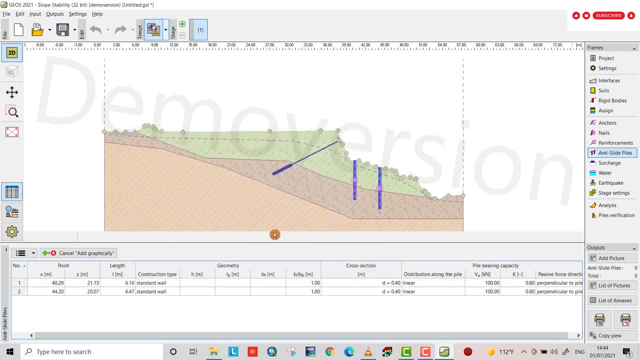 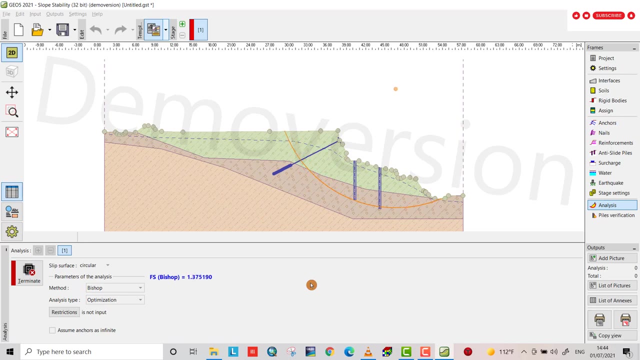 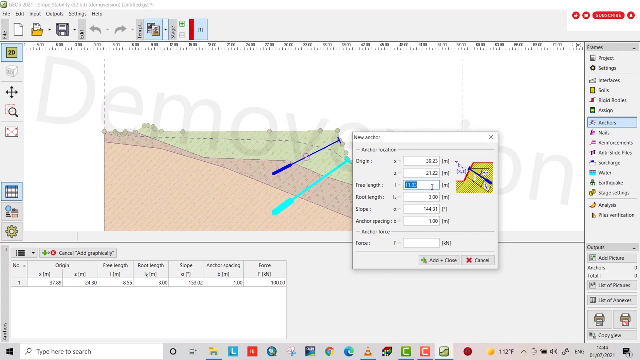 d: 1 meter, 100 and 0.8. okay, analyze. so it's still not safe. 1.35 is not safe. so what should we can do? we can provide another anchors screen meter and it became 100 kilonewton. okay, this time analyze. 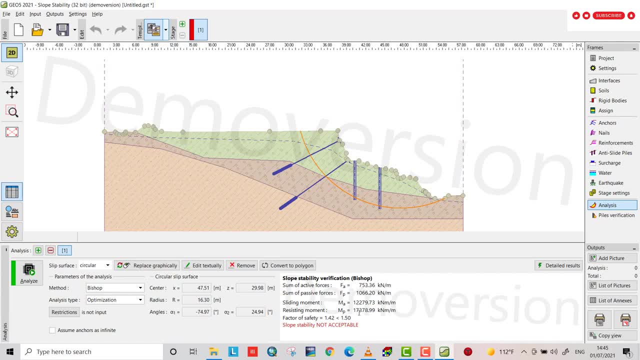 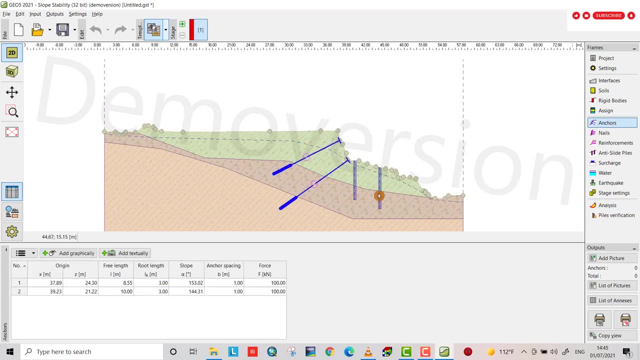 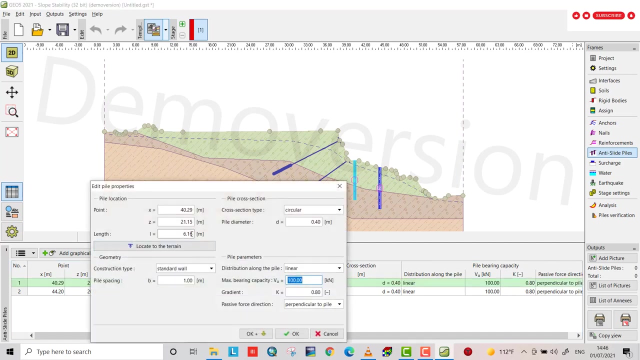 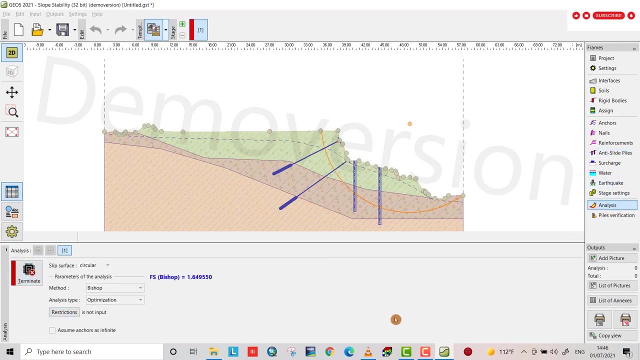 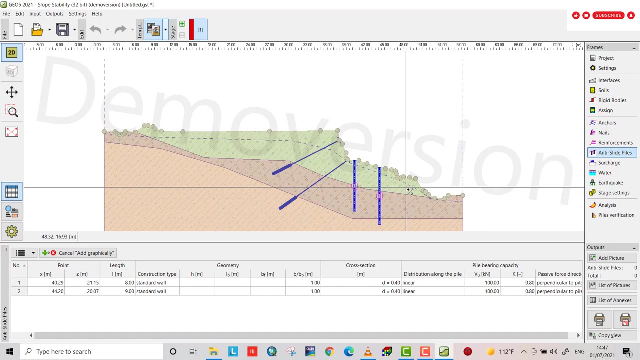 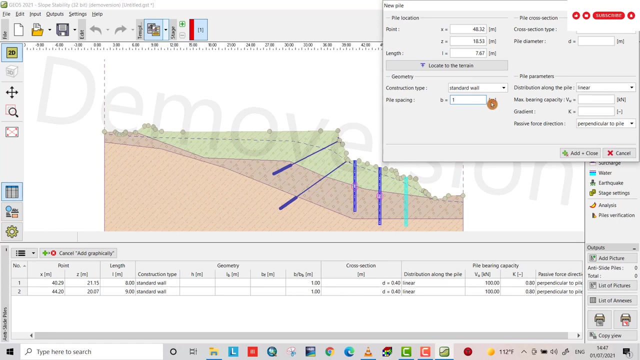 142. it is uh near to the limit, so you can provide another anchor or change- sorry, or change is the language. if eight, okay, nine, okay, analyze you, almost a, it's almost, let's change and more. let's provide another anti-slide pile here. okay, one meter, 100 kilonewton and 0.8. 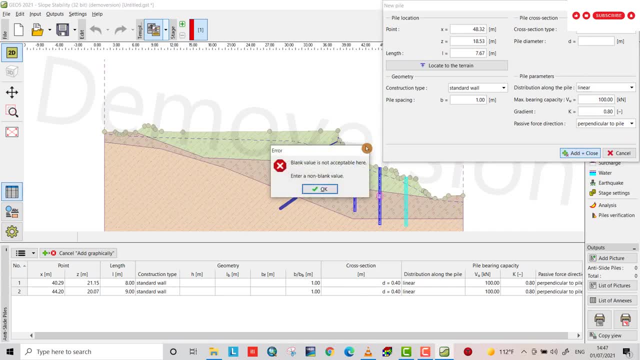 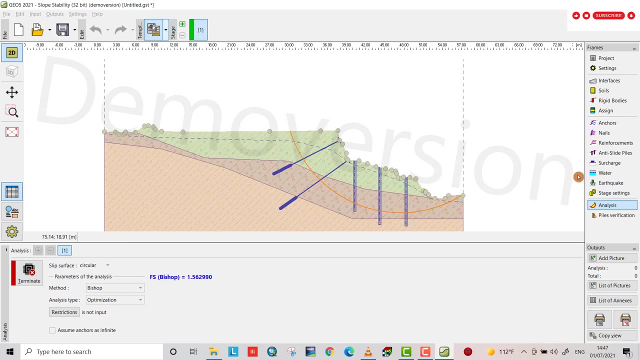 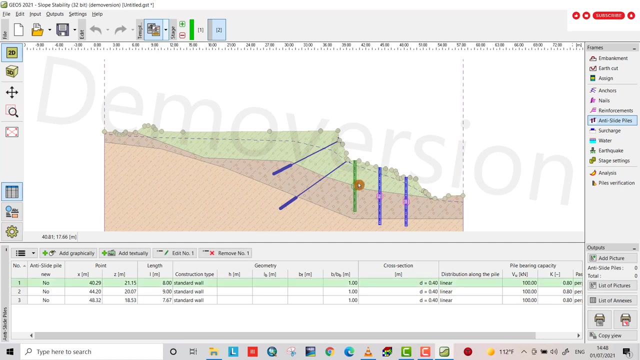 the okay, sorry, 0.4. okay, analyze time you. okay. now we just say: now we can say it is provide another stage for the stage we can change the anchors and Nellis, anti-slide pilots. okay, I remove this. is this. yes, I don't need this one, sorry. 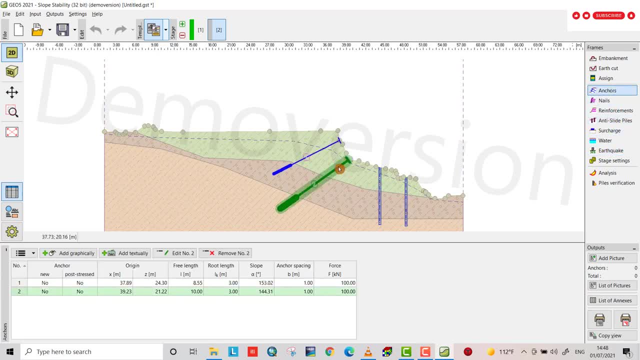 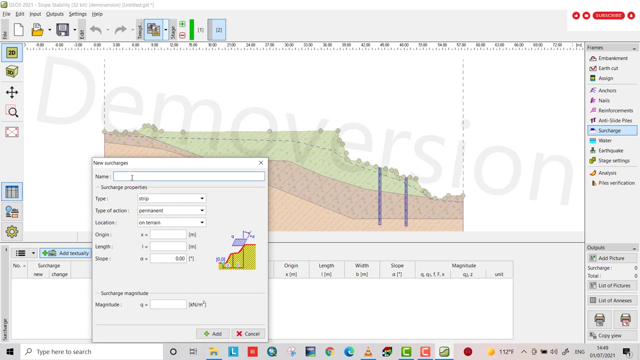 anchors, yes, remove also. I try. I want to provide safe charge. I text only how is for them to be? have a house the trip, yes, permanent on Terrain x, from where, if we have here from 21, from 24, ok, from 24, and language, is he sick meter? 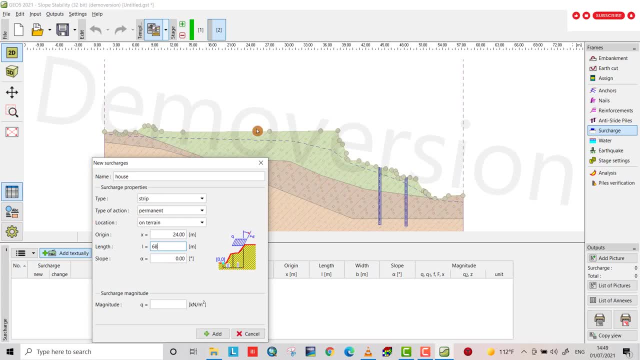 or a bit of speed change to this name here: x1, prostate, francx, from 28, from 25, u and k is called x and then the et pre, Or 8 meter, Sorry, 8 meter Alpha. okay, And the magnitude it will be 100 kilonewton per meter squared. 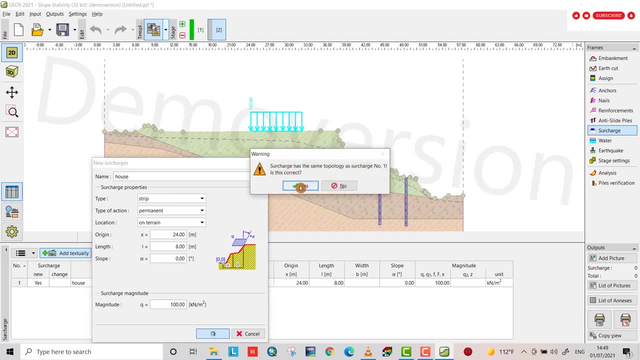 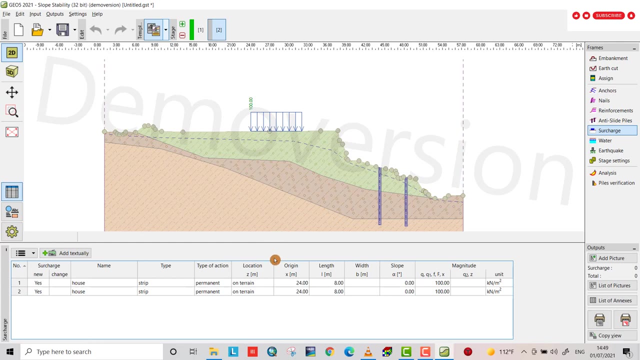 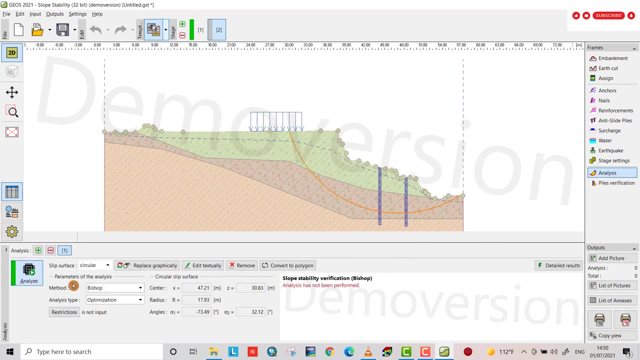